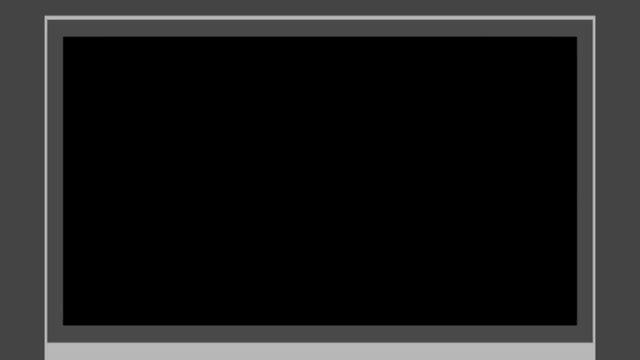 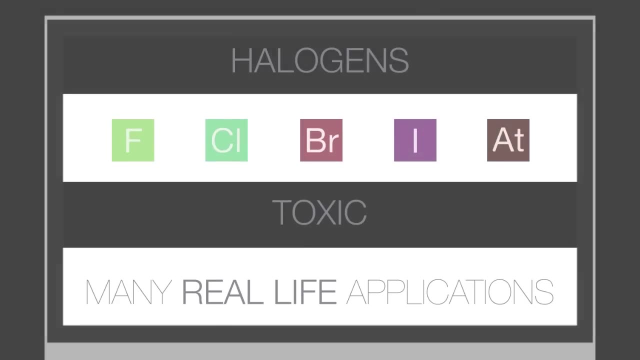 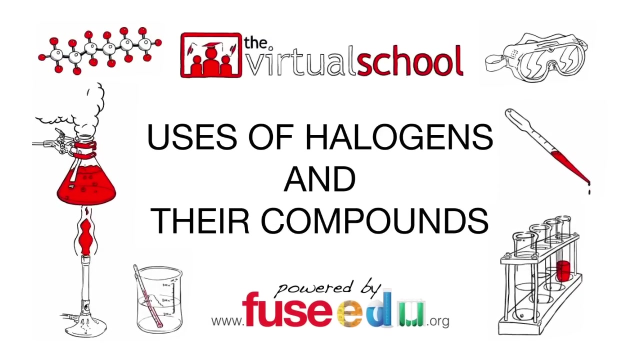 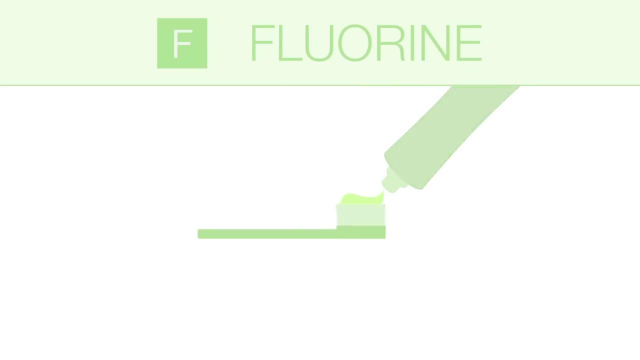 We have mentioned before that halogens in their elemental form are toxic. However, their compounds are, in fact, very useful and used in everyday life. In this lesson, we will learn about the many uses of halogens and their compounds. When you woke up this morning, you likely brushed your teeth. Toothpaste usually contains sodium. 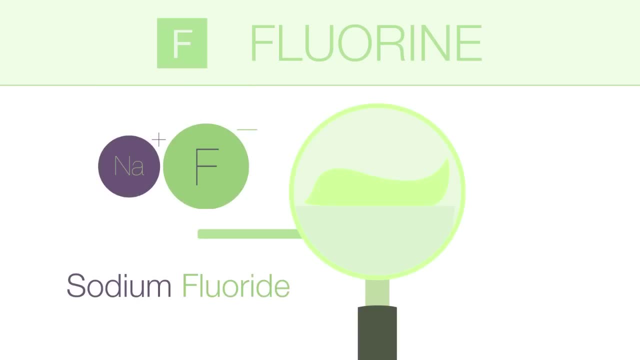 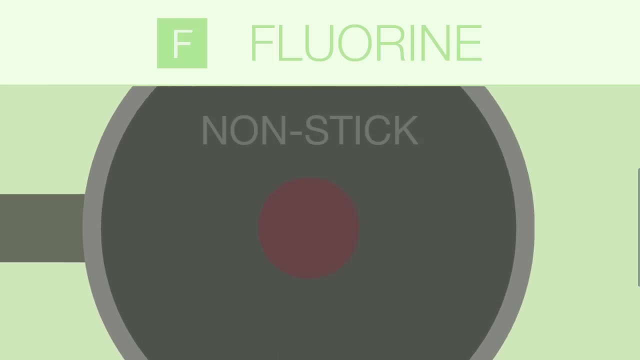 fluoride, which acts to prevent tooth decay. For the same reason, some countries fluorinate their water supply. Some of you may have decided to have a fried egg for breakfast and may have used a non-stick pan. The reason why the pan is non-stick is due to a layer of teflon. 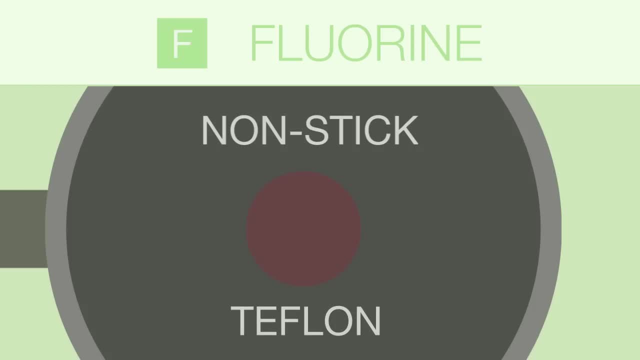 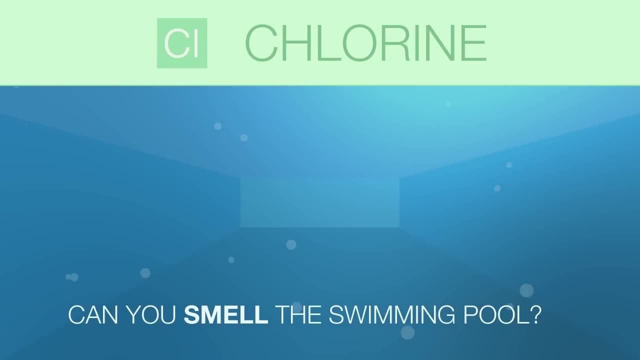 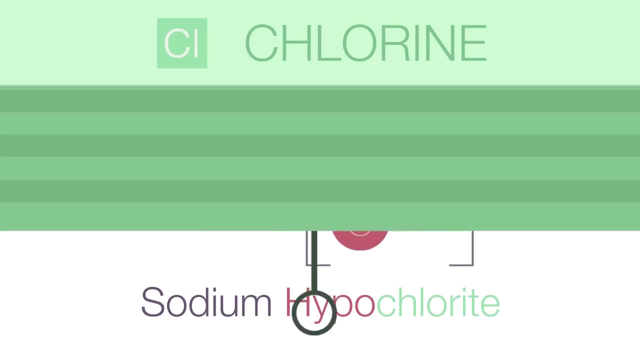 a fluorine-containing compound. Let's close our eyes and think about a swimming pool. Can you smell the swimming pool? That smell is, in fact, because of a chlorine-containing compound, sodium hypochlorite. Now let's change the scene just a bit. Imagine you have been asked to do some chores. 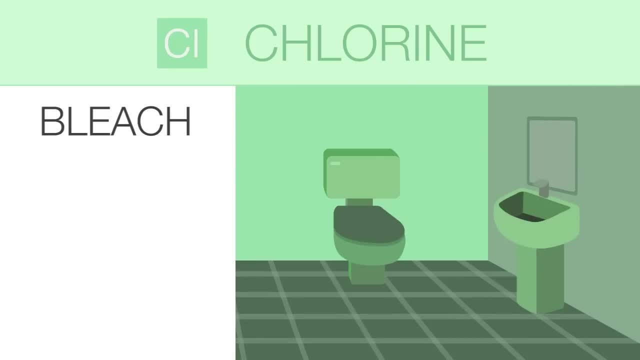 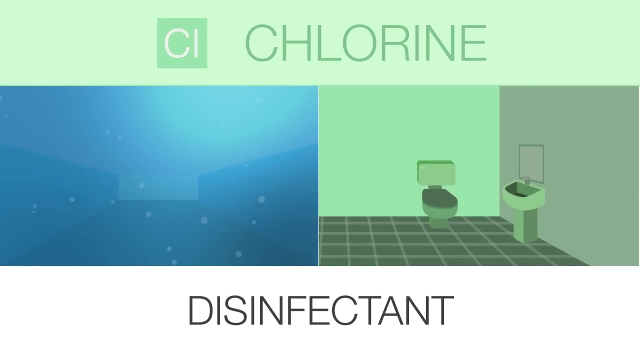 cleaning the bathroom sink and toilet. Bleach, which is a common household cleaner, is also a solution of sodium hypochlorite. In both cases, sodium hypochlorite acts as a disinfectant, In other words, it kills germs. Many countries chlorinate their water supply as a disinfectant. 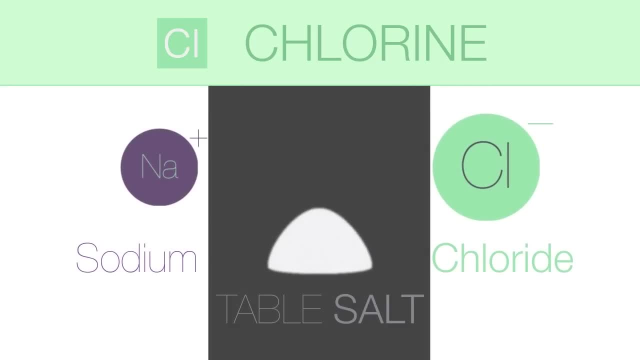 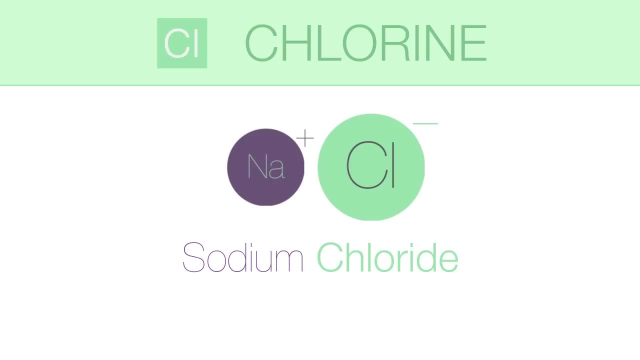 measure. Regular table salt is sodium chloride, As you know very well. it is a flavoring agent and enhances the taste of food. If you live in a cold climate, you may have had to salt the pavement of your driveway prior to an anticipated snowstorm. Road salt is a very common ingredient. It can be used. 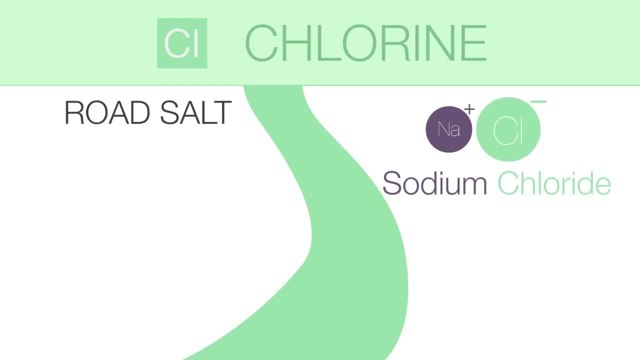 in a lot of different ways. For example, if you live in a cold climate, you may have had to salt the pavement of your driveway prior to an anticipated snowstorm. Road salt is a mixture of sodium chloride and calcium chloride. The sodium and calcium chloride solution that